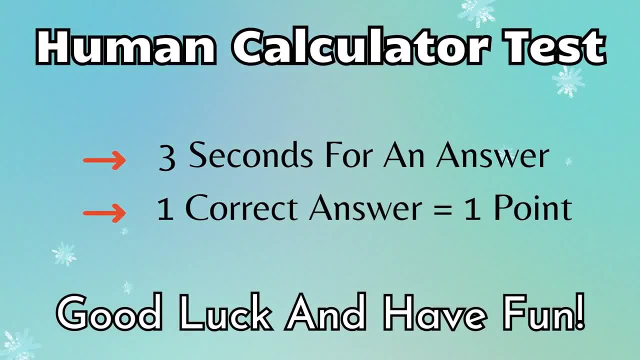 Welcome to the new Puzzle Monster video. In today's video we are going to check if you are a human calculator. Be quick, because you will get only 3 seconds for an answer. There are 40 questions and you will get 1 point for each correct answer. 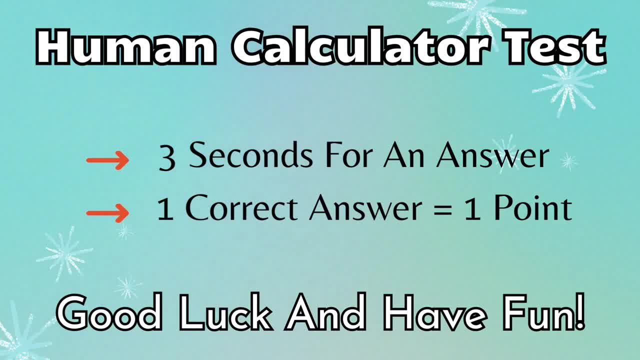 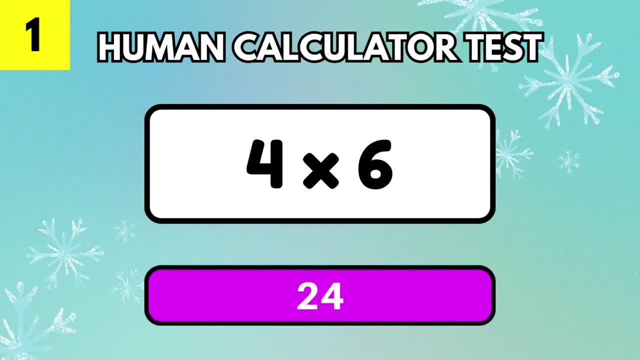 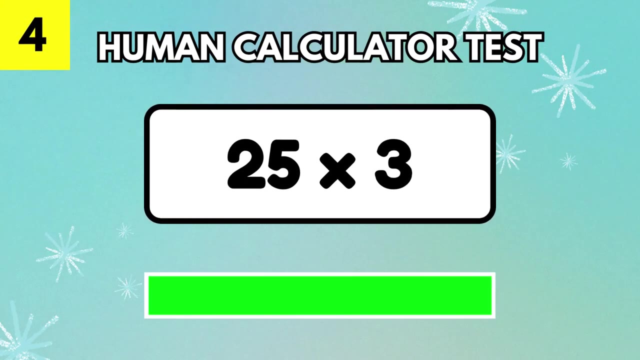 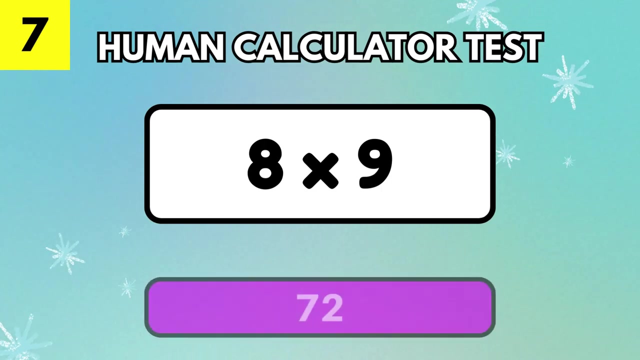 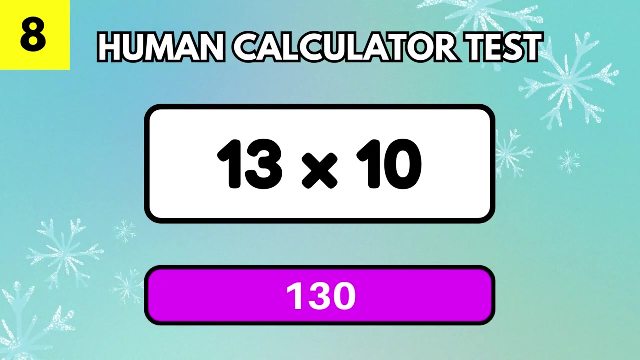 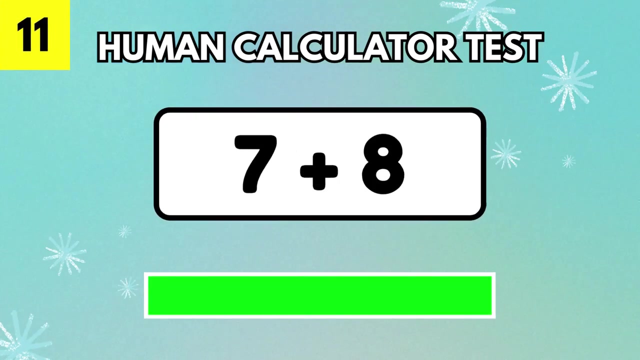 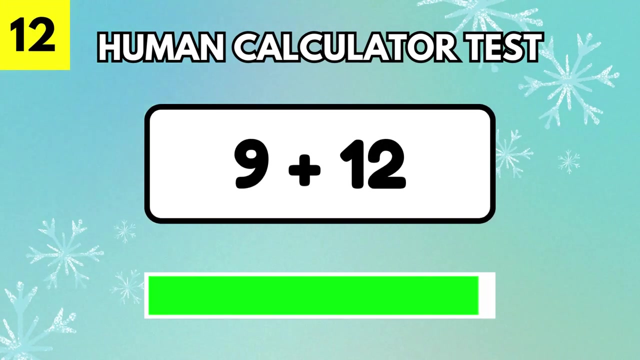 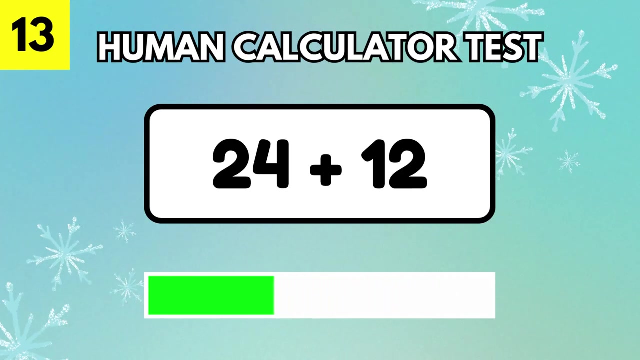 Comment your score at the end of the video. Good luck. 35, 88, 75, 64, 144, 72, 130, 45, 180, 15, 18, 19, 20, 21, 21, 36, 36, 46, 44. 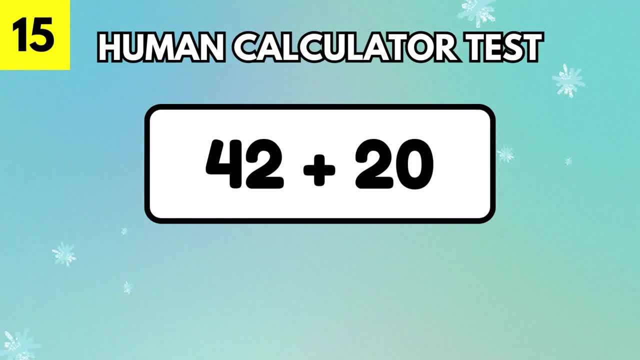 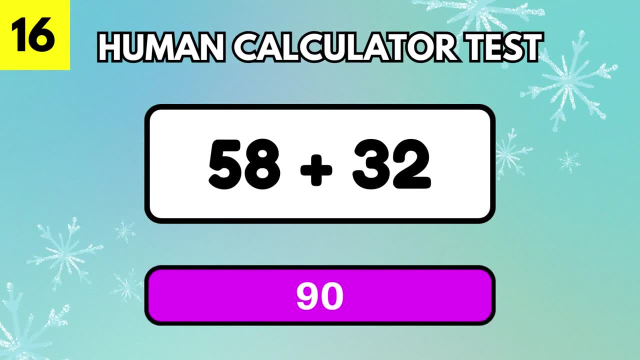 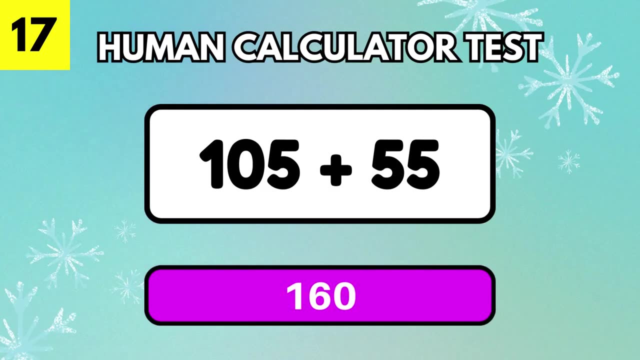 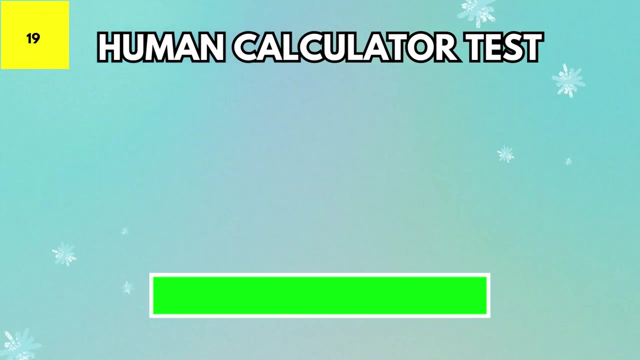 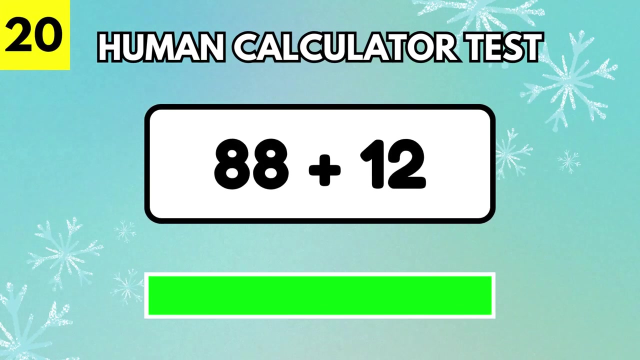 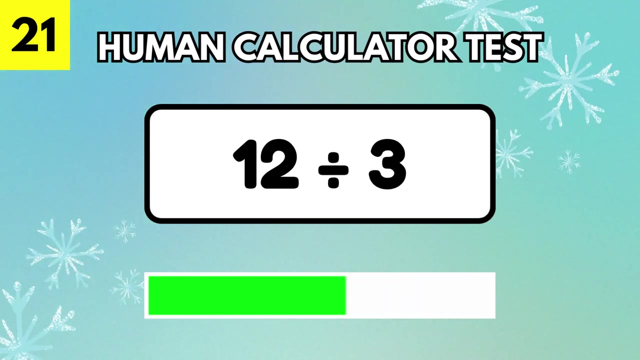 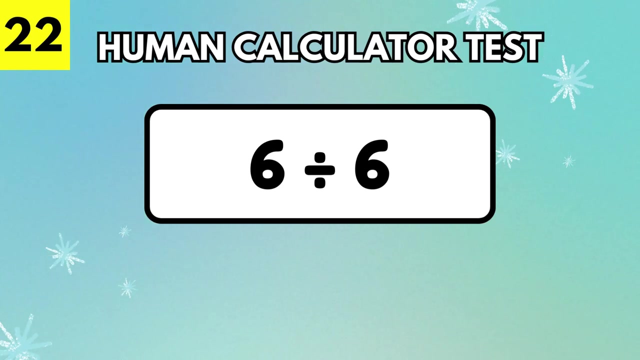